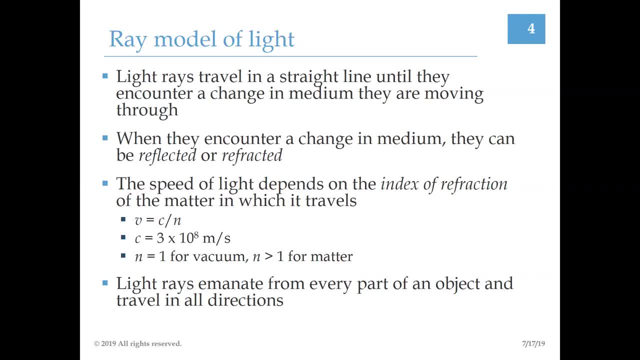 until the medium in which I'm moving through changes. So if I go from air to water or water to glass, for example, at that point that is a change in medium And that's going to cause me to change the direction in which I'm moving. 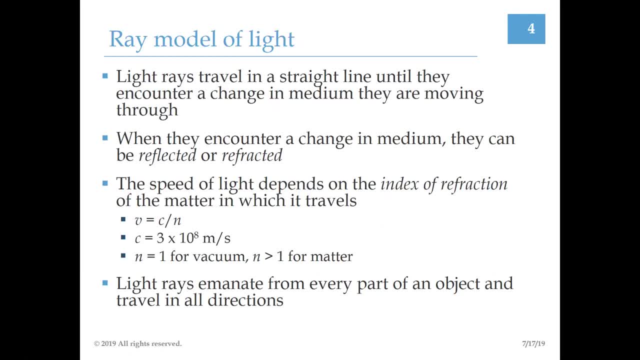 So, specifically, when you encounter a change in medium, as a beam of light, you can either be reflected or refracted. We'll define those in a slide or two here in the future. Now, the speed at which the beam of light travels will depend on a property of the material that it's in, called the index of refraction. So in a vacuum. 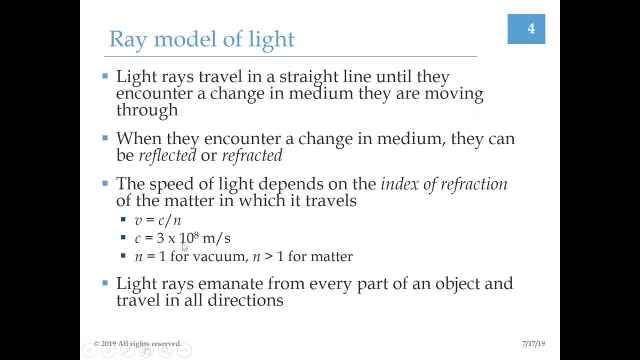 the speed of light has this value of three times 10 to the eighth meters per second. So when people talk about the speed of light, that's what they're referring to. That's the speed of light, And we use the little letter c to represent the speed of light. 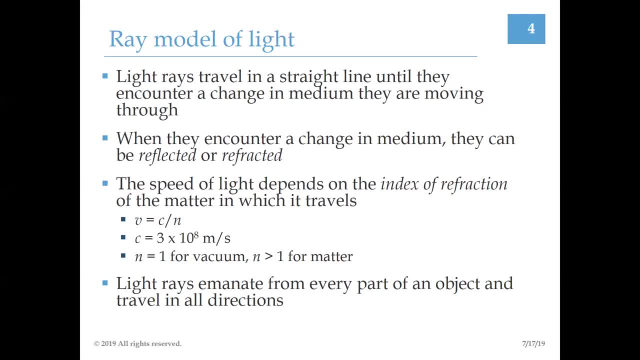 Now, if I happen to be moving through something that's not a vacuum, then what I'm going to do to figure out the speed of light in that material is to take this constant of three times 10 to the eighth meters per second, and I'm going to divide it. 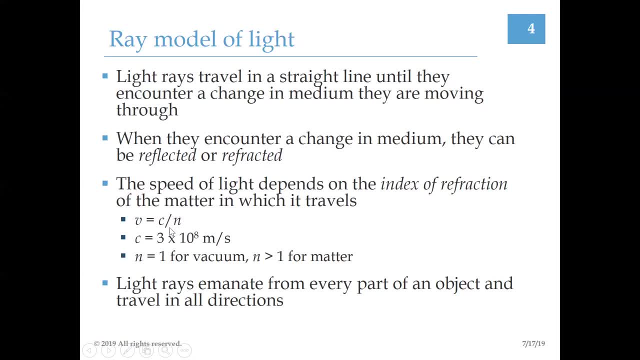 by the index of refraction of the material. So n here represents the index of refraction of the material. n is always a number that is either equal to one or it's greater than one. So n will be equal to one for a vacuum. If you're dealing with something that is not a vacuum, n is going to have a value that's greater than one. For air, you can approximate the air that's surrounding us as a vacuum. It turns out the index of refraction for air is 1.1.. 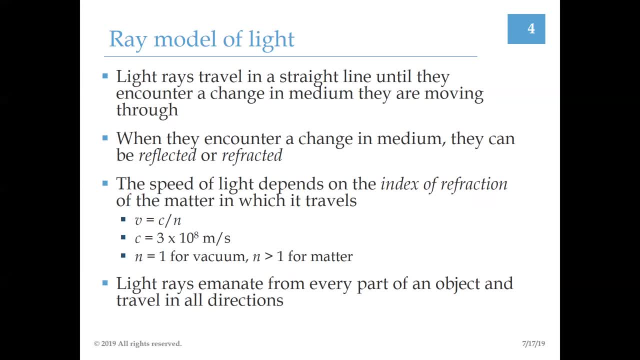 And then there's some non-zero digits kind of way out there, but it's pretty close to a vacuum. So for air we can use n equals one. The other thing about this model is we have to imagine that an object that's giving off light is emitting these light rays from every part of itself and they're traveling in all directions. 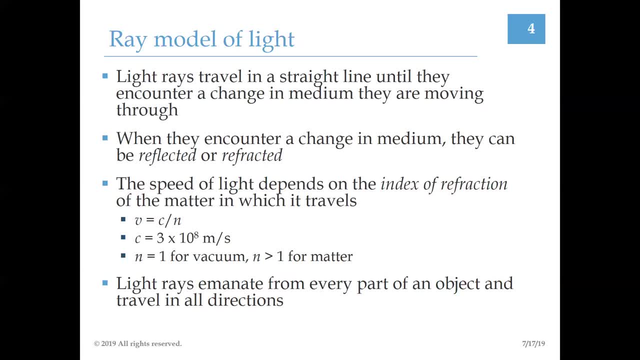 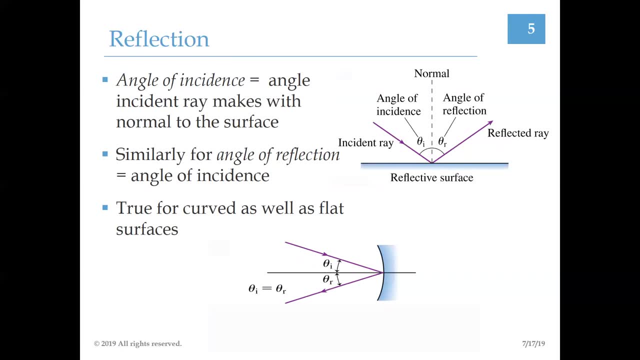 So this is the ray model of light And let's see how we can actually build upon this model to understand the behavior of light. So the first thing to talk about is reflection, And the thing about reflection is it's actually the simple of the two cases. So take a look at the. 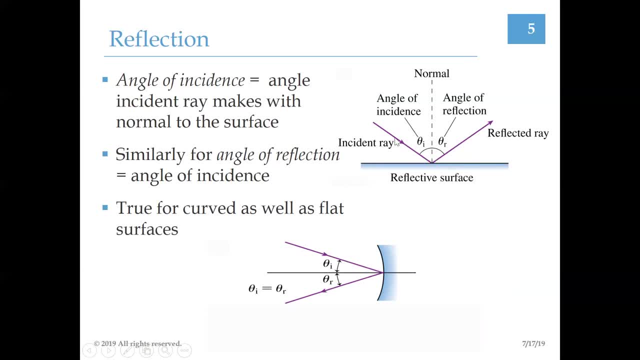 drawing that we have here on the left. We've got some beam of light that's coming in towards the reflective surface. This beam of light that's coming in, that's called your incident ray. I know kind of our common everyday vernacular speak. an incident sounds like this ominous event. 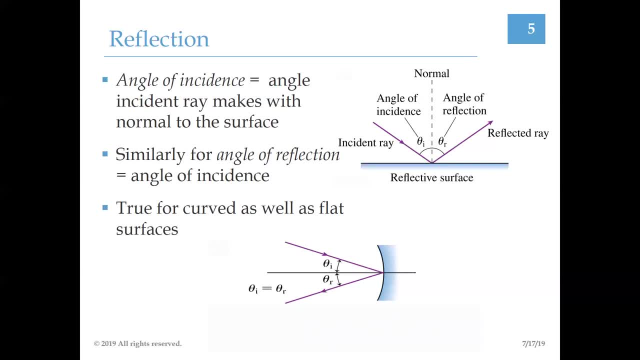 That's not what we mean when we use the word incident here. in optics, Incident just means the beam of light that's coming in, the beam of light you start with. So your incident ray comes in, it hits this surface and it gets reflected off. 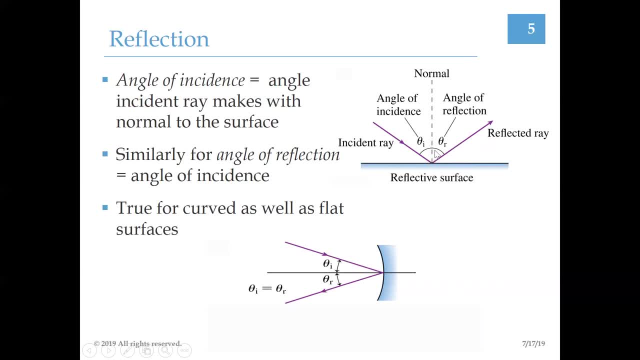 Now we're going to draw a line here that is perpendicular to that surface, And it's represented by the dashed line here That is called the normal. So normal just means perpendicular. We've actually encountered this before in physics when we talked about normal forces. This is not a force, it's just an imaginary line that we've drawn. 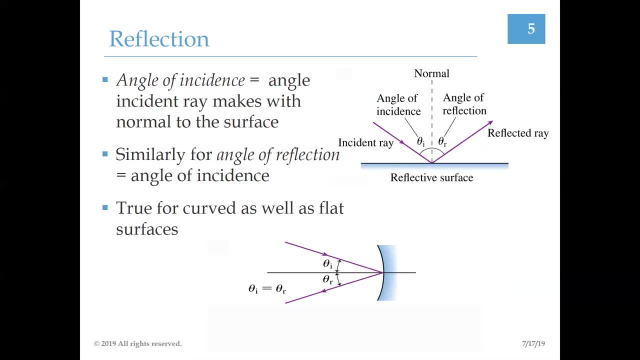 The normal line is always going to be perpendicular to a surface, at whatever point we're talking about. So notice, we've defined a couple of angles here. One angle is called the angle of incidence. The angle of incidence is the angle that the incident ray makes with respect to the normal. 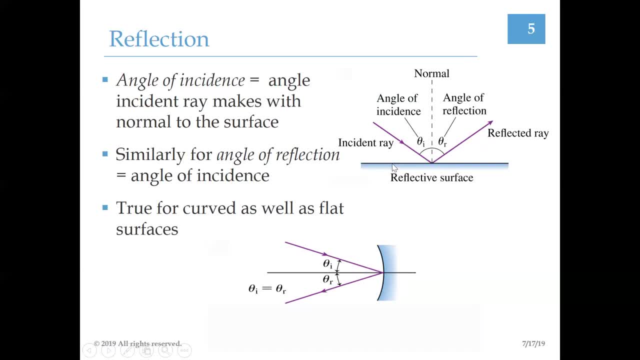 It's not with respect to the point, the reflective surface itself, It's with respect to the normal. That's something very important to keep in mind when we're talking about optics- All of the angles you're going to deal with in optics here. 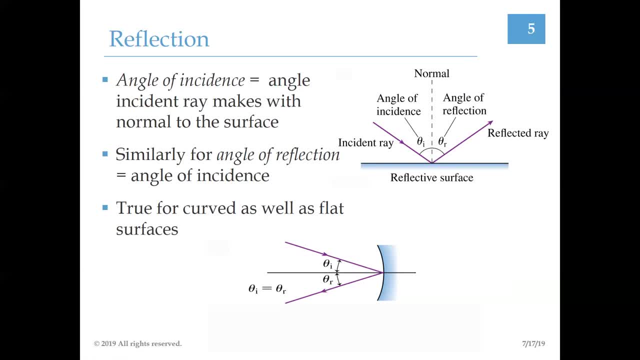 are always gonna be measured with respect to that normal line. Likewise, you can define an angle of reflection measured between the reflected ray and that normal line, And for reflection, that angle of incidence will always be equal to the angle of reflection Period. full stop, end of story. 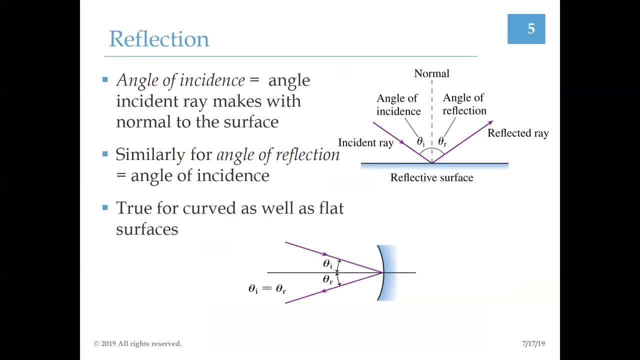 Those two angles are always equal to one another. This is true for flat surfaces and curved surfaces as well. So at the very bottom here we are showing an incident ray hitting some curved surface and the reflected ray that comes off of that surface. Notice that we've drawn in that solid black line. 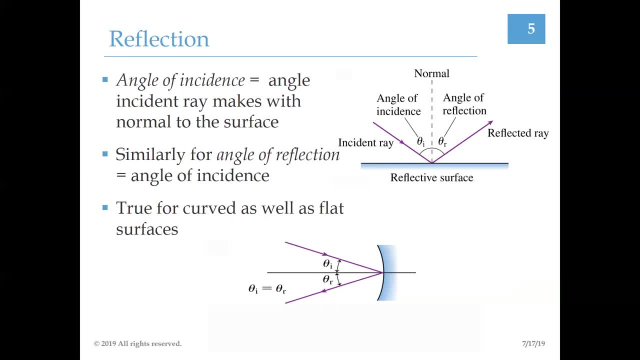 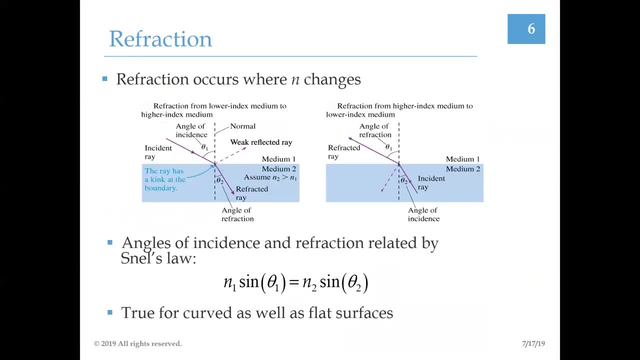 That is the normal to the surface. at that point, And as expected, the incident and reflected angles are exactly equal to one another. So refraction is a little bit more complicated than reflection. So refraction occurs when the beam of light actually passes through into the new material. 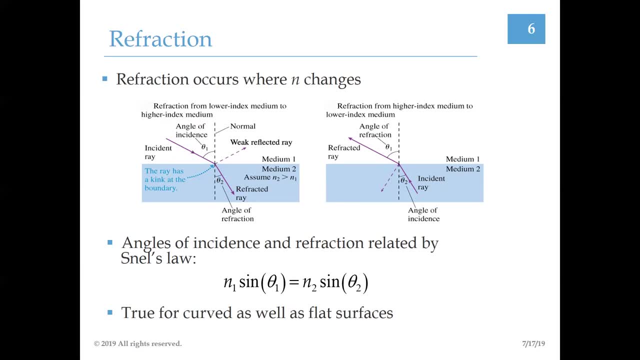 So instead of being reflected off, instead of bouncing off the surface, it actually passes into the new material And when that happens, the ray of light is gonna get bent. So when you hear refraction, think of the ray of light gets bent compared to the direction. 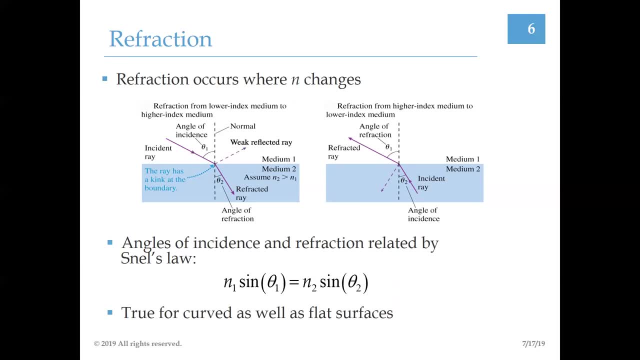 in which it was originally moving. So we can define some angles here. Once again, we can define an angle of incidence as the angle between the normal to the surface and the incident ray, And we can also define an angle of refraction which, as you might expect, 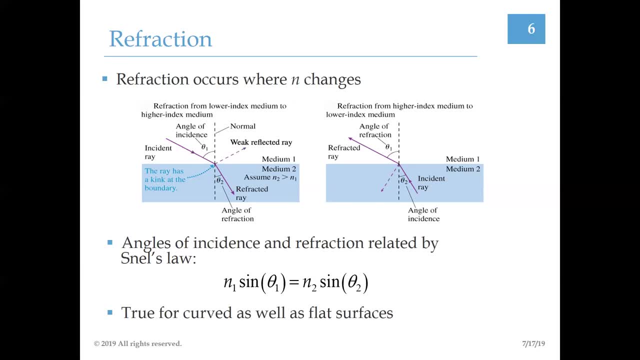 is the angle between that normal line and the refracted ray. Notice something that incident: beam of light is always going to be on the opposite side of the normal from your refracted ray. So here, in both cases, we're showing here your incident. 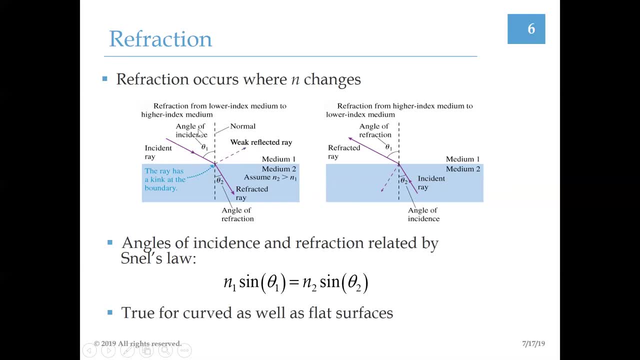 ray on the left-hand side is on the left of the normal. Your refracted ray is on the right. In the other diagram, the incident ray is coming up from the bottom, so it's on the right side and then your refracted ray is on the left. 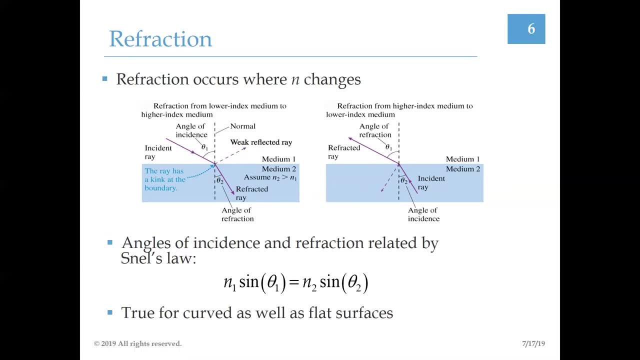 The angles of incidence and refraction could be related to one another by Snell's law. Before you email me saying, hey, you've misspelled Snell in the textbook, there are two L's with Snell. In fact, when I Google this on Wikipedia and everywhere on the 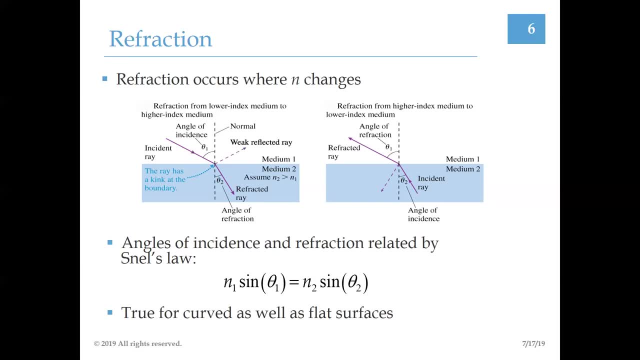 internet. there are two L's in Mr Snell's name. It turns out everybody's wrong. One of my colleagues who's actually done a little bit of looking to the historical record turns out Mr Snell actually spelled his name with one L. Over time it seems to have accumulated an extra L, but that was not. 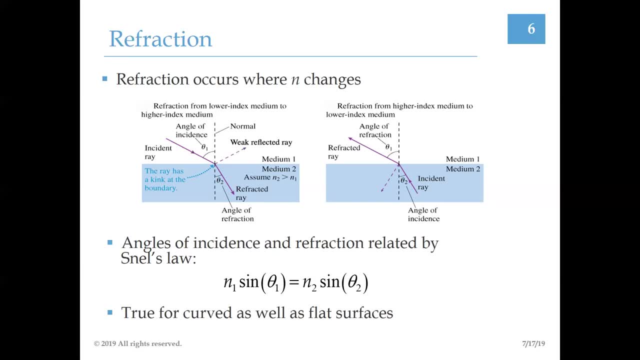 something that Mr Snell did to his own name in his lifetime. So, as somebody who has a name that people like to insert all sorts of extra L's into, I'm going to respect Mr Snell's decision and we're going to write it with just one L. 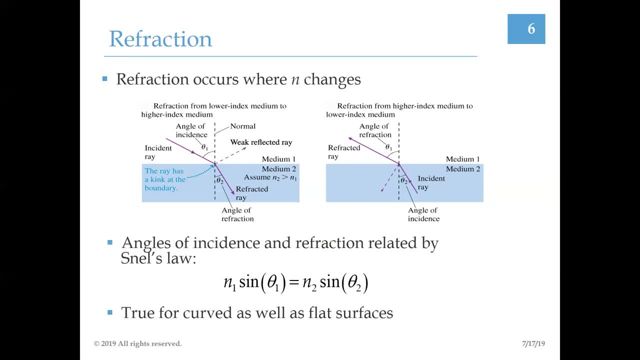 With that little bit of historical aside out of the way, Snell's law basically says: okay, take the index of refraction for one medium and then use the angle that the light makes in that medium. It could be the angle of refraction or the angle of. 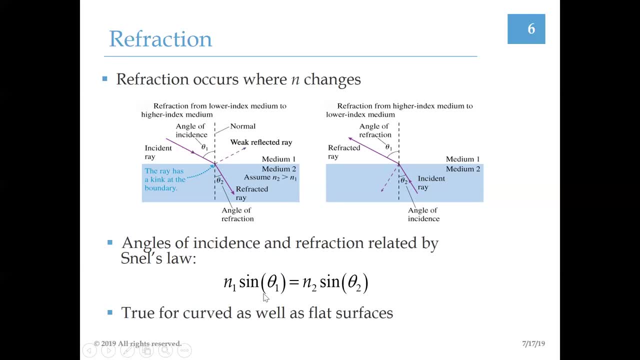 incidence. So n1 sine of theta 1. And then that's going to be equal to the same quantity for the other medium, n2 sine of theta 2.. So the 1 refers to one medium, the 2 refers to a different. 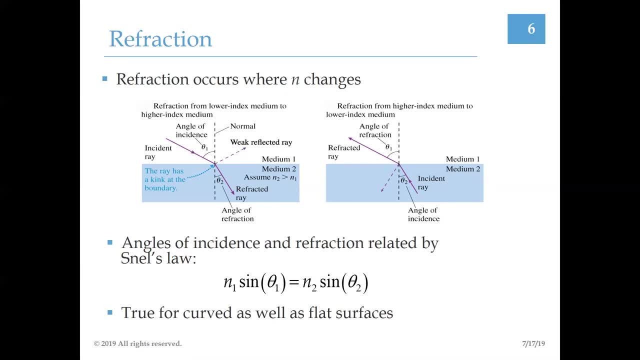 medium. So know your index of refraction for both media, measure your angles in both media, and Snell's law will always hold true. And once again, this is going to work for both flat and curved surfaces. Okay, with that in mind, I've 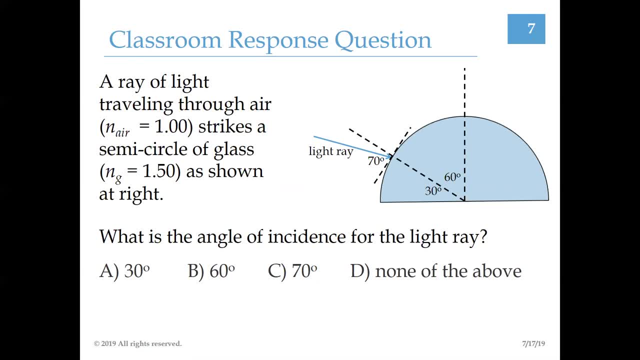 got a question for you. Please go ahead, pause your recording, read this question and we'll get back to you. Make sure to submit your answer to Gradescope. The correct answer for this question is actually D, none of the above. So remember the angle. 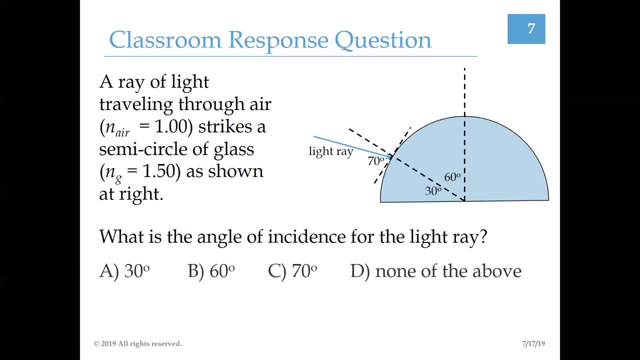 of incidence is defined as the angle that the incident light ray is going to make with respect to the normal. So if you take a look at the diagram we have here, this light ray is going to be hitting this curved surface, and right at the point that it's going to 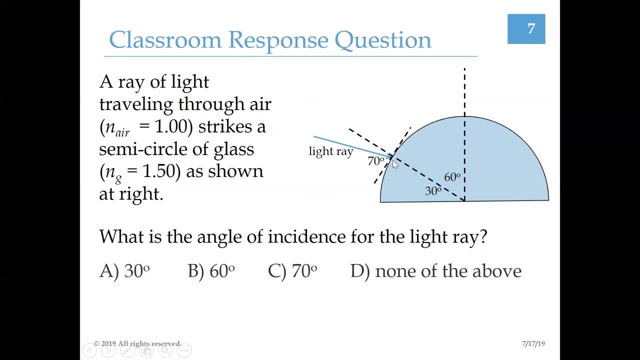 hit. we've sketched in a tangent line to that surface and a normal line to the surface, And so we're told that the light ray makes an angle of 70 degrees with respect to that tangent line. Well, the tangent line and the normal line have to be perpendicular to one. 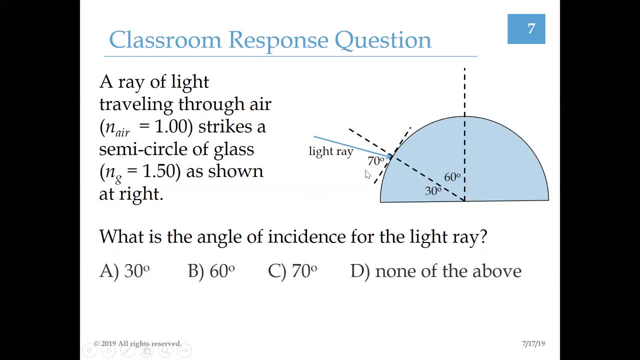 other. So that total angle is 90 degrees. So if I've already used up 70 here, that means I've only got 20 degrees left for the angle between the normal and the incident ray of light itself. So the correct answer here is D. none of the above, because the 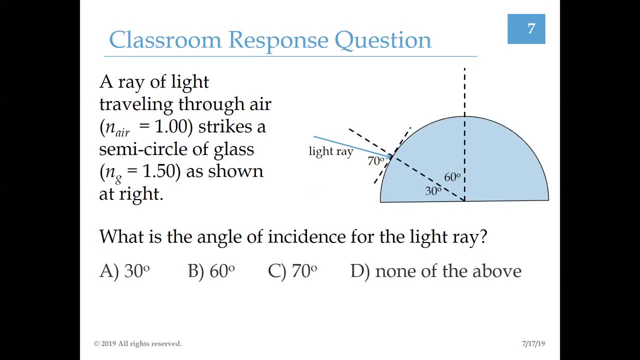 angle should be 20 degrees. Here's another question for you. Please go ahead, pause your recording and submit your answer to Gradescope. The correct answer to this question is B, 20 degrees. Now some of you may be wondering. 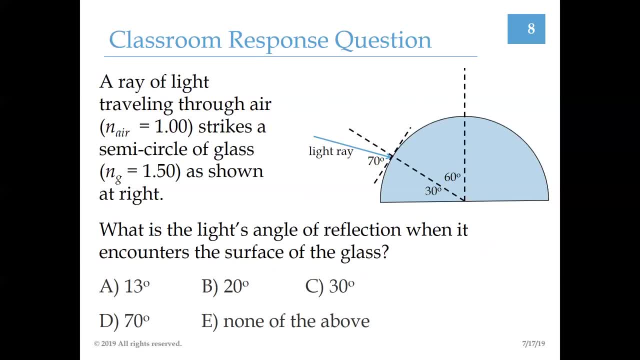 wait, I calculated a different number than 20 degrees. How did you get 20 degrees? Notice, the question is asking about reflection, not refraction, Refraction: if we're dealing with refraction, then you'd use Snell's Law, But Snell's Law does not apply to reflection. For reflection: 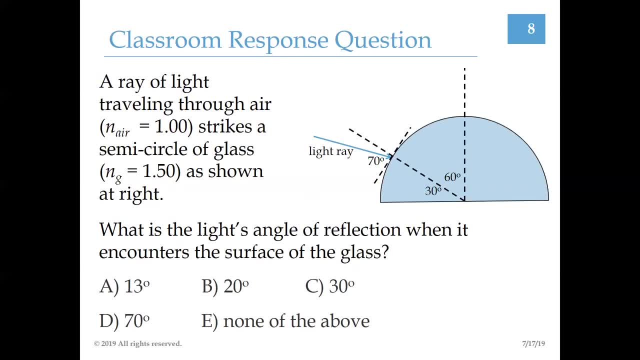 remember, the angle of incidence is equal to the angle of reflection. So we just figured out the angle of incidence. on the previous slide It was 20 degrees, So that means the angle of reflection must also be 20 degrees. So some of this light is going to hit the 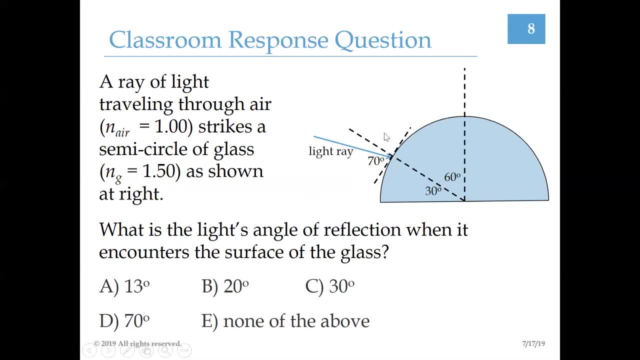 curved surface here. Some of it will bounce off, Some of it will be reflected, Some of it will pass through and be refracted. That's actually pretty typical Whenever a light encounters a new medium. a portion of it will be reflected and another portion will be. 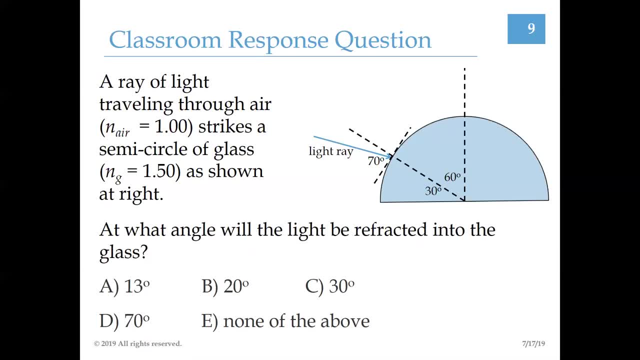 refracted. So, with that in mind, here's the question I think you've been waiting for All right. Now that you've had the chance to pause your recording, I'm going to turn you back to the Q&A, All right. 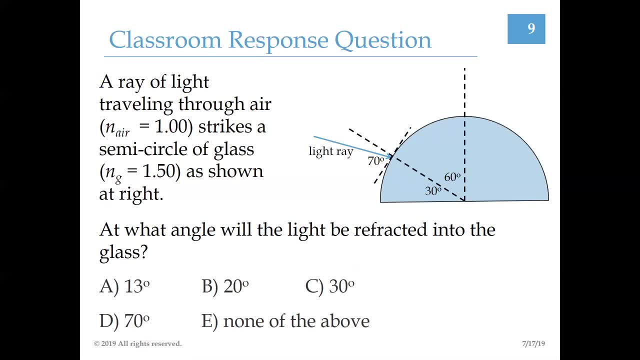 Thank you. All right, Let's get back to our Q&A- All right reporting and submit your answer to Gradescope. I'm going to reveal the correct answer. The correct answer here is A, 13 degrees, And again, we're just applying Snell's law to calculate that. So 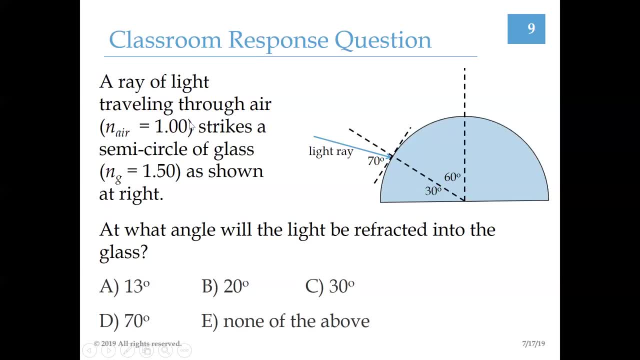 we know the index of refraction of air pretty close to one. We'll approximate it as one. We know the index of refraction of glass: 1.5.. We know the angle of incidence is 20 degrees. So we can plug all this into Snell's law and figure out the angle of refraction is 13 degrees And 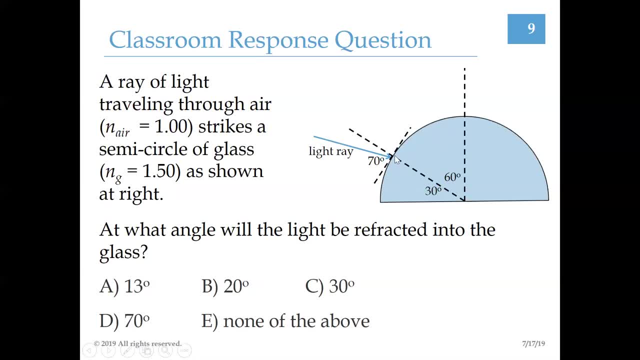 again, don't forget that angle of refraction is going to be defined as 13 degrees with respect to this normal line here. So we're going to come out to the right of the normal line and we're going to make an angle of 13 degrees with respect to the normal line. 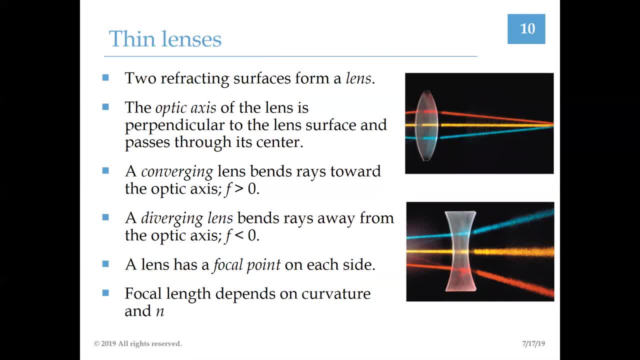 Okay, so once you understand the basis of refraction, we can start talking about lenses. So if I have two refracting surfaces, those two refracting surfaces constitute a lens, And so this could be something as simple as maybe the lenses in your glasses. It's something as complex. 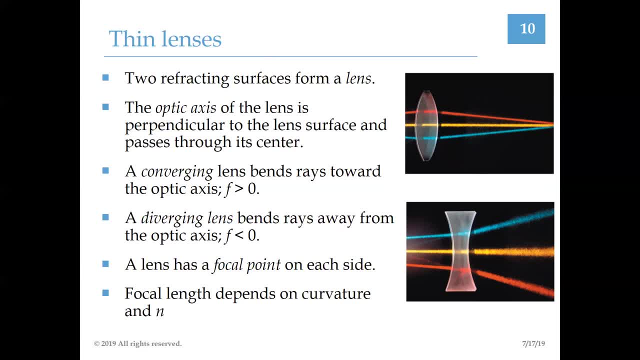 as maybe the lens of a telescope or a microscope. Actually, when you get down to it, those two really aren't much more or less complicated compared to one another, at least to the degree we'll be talking about them. So I've got a few more terms I need to introduce you to here. 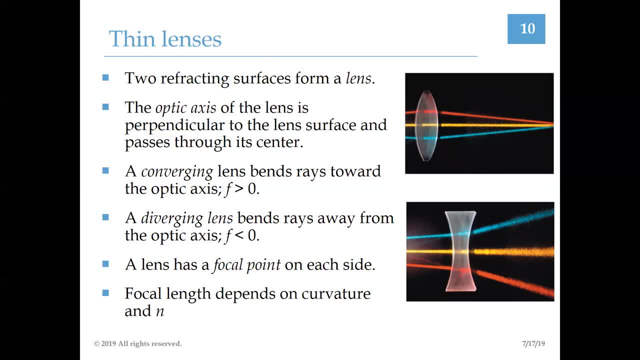 The first is called the optic axis. The optic axis is just a line that is perpendicular to the lens and passes right through its center. So if you look at the pictures we have here, we've got a beam of red, a beam of yellow and a beam of blue light in each of those pictures. 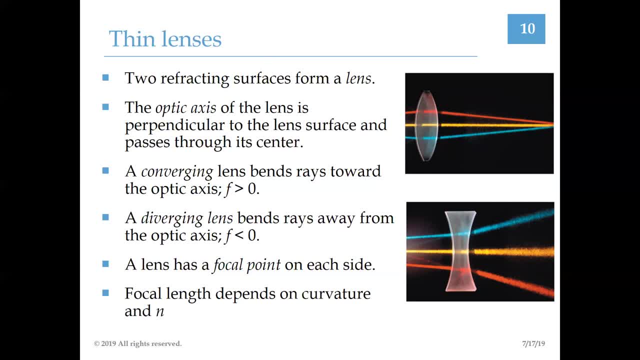 The yellow light is going to be the one that's falling along the optic axis. It's perpendicular to the surface of the lens and it's passing through the center of the lens. Now, those two lenses that we're showing there, they're actually going to be the lenses that we're. 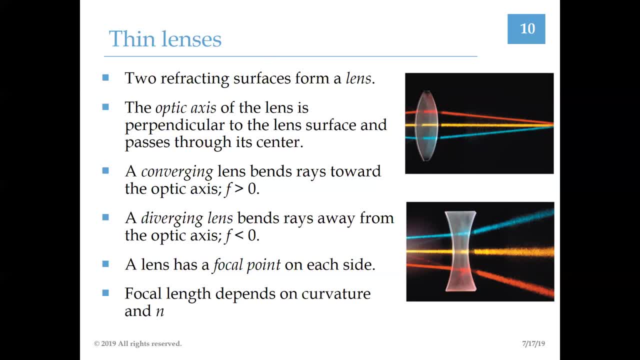 going to be using. They're actually two different types of lenses, So, in general, all lenses are either going to be converging or diverging lenses. A converging lens is going to be a lens that bends light toward the optic axis. That's what we're showing in the top diagram here. This is a 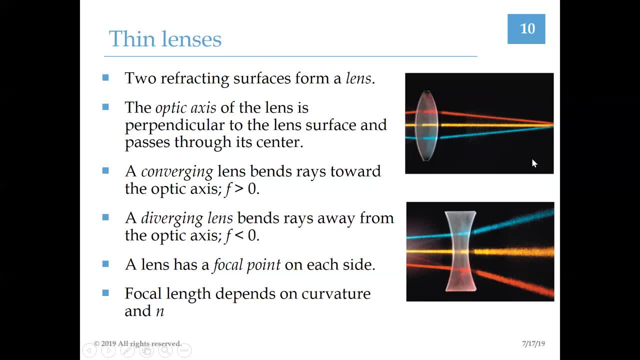 converging lens. The light rays converge towards one another. A diverging lens has rays of light that, after they hit the diverging lens, are going to bend away from the optic axis. That's what we're showing here in the bottom picture. 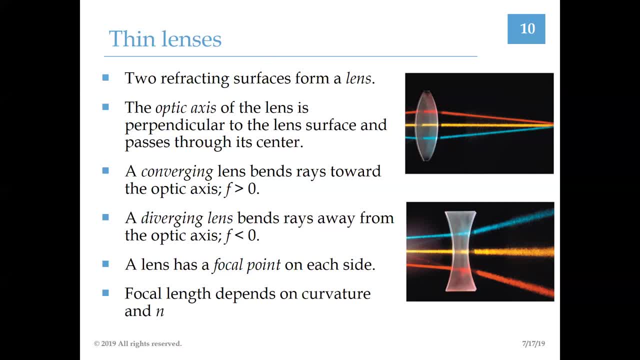 Lenses have a property called a focal length. We represent it by the letter F. We'll be talking some more about focal length here in a few slides. For right now I just want to put a placeholder in your mind: If you have a converging lens, the focal length will always be positive. 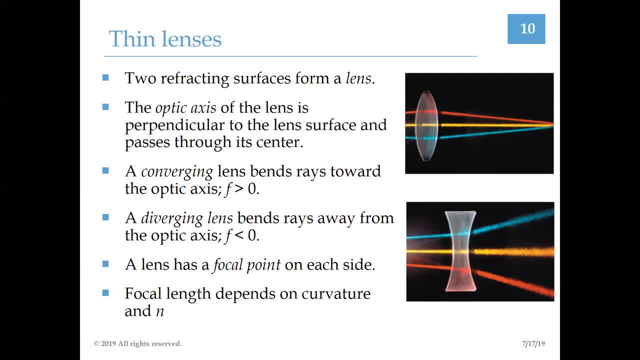 If you have a diverging lens, the focal length will always be negative. Now a lens is going to have what we call a focal point on each side of the lens And again I haven't really defined that yet. You're going to see what that looks like graphically here in a couple of slides, But just 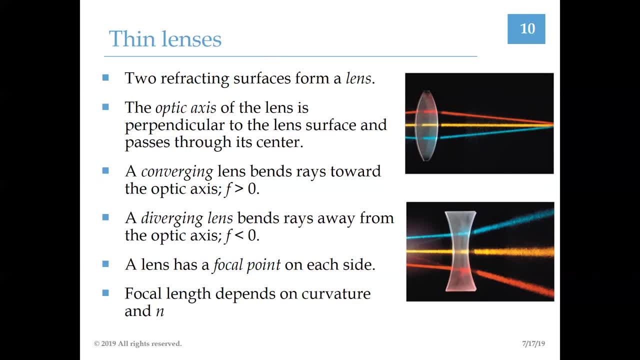 know that the focal length and the location of those focal points is going to depend on the curvature of the lens. So how much the lens is curved and the material you make it out of, In other words, it depends on the index of refraction of that material. 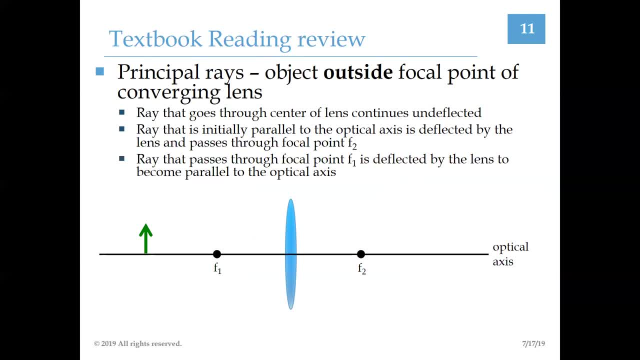 Okay, so at this point we're going to do something called ray tracing. So when you've got an object that's emitting light, you could, if you wanted, to apply Snell's law to every bit of light that comes off that object that happens to hit your lens And you could use Snell's law to then figure. 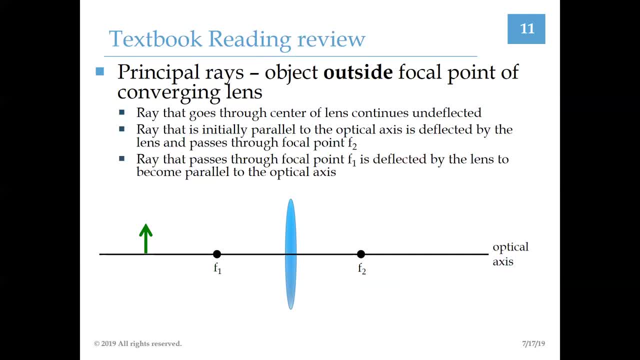 out how those beams of light are going to behave after encountering the lens. But we can actually take a little bit of a shortcut. We can do something called ray tracing. And with ray tracing, what we're going to do is we're going to draw three what we call principal rays. These principal 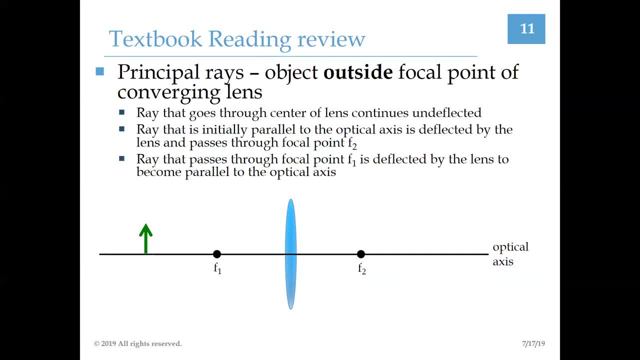 rays are rays that actually make it easy to figure out what's going on after the light from the object passes through your lens. So ray tracing is definitely a skill that you're going to be practicing today and in studio today, and you will also need to be able to do it on the exam. So let's 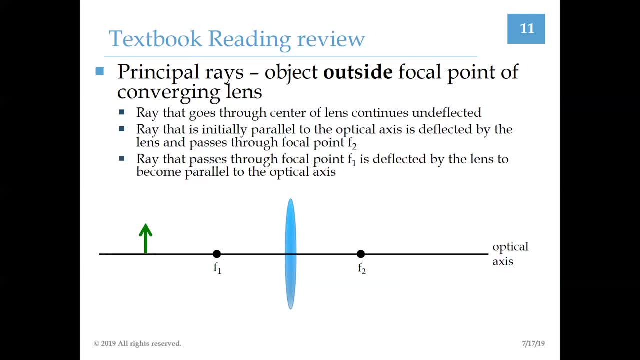 take a look at the next slide. So let's take a look at the next slide. So let's take a look at the next slide. look at this case. right here We have a converging lens, So this blue oval here represents our 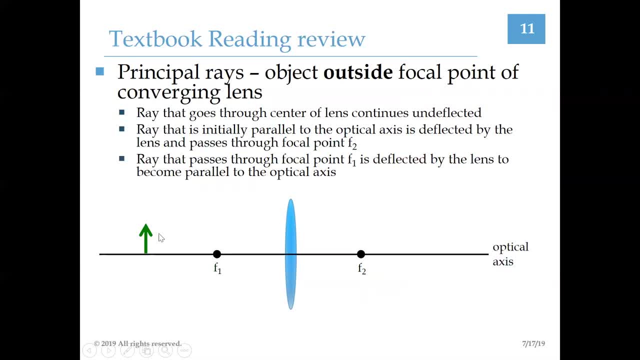 converging lens. This green arrow here represents the object And I've placed the object outside of the focal point of the converging lens. So F1 and F2, that represents the focal point of the converging lens. Each focal point is one focal length away from the lens, So focal point one is 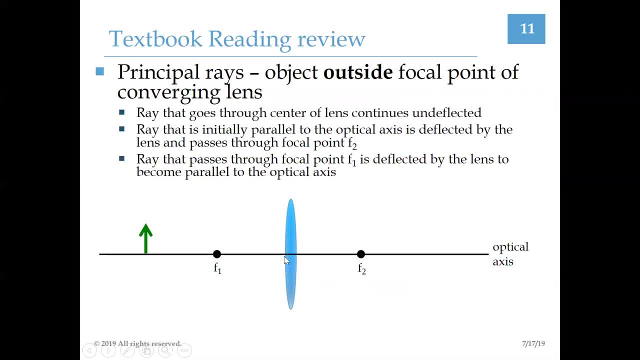 a focal length: one focal length to the left of the lens, Focal length to the focal point. two is one focal length to the right of the lens. So once you know the focal length, once you're given that value, you know the location of the two focal points relative to the lens. 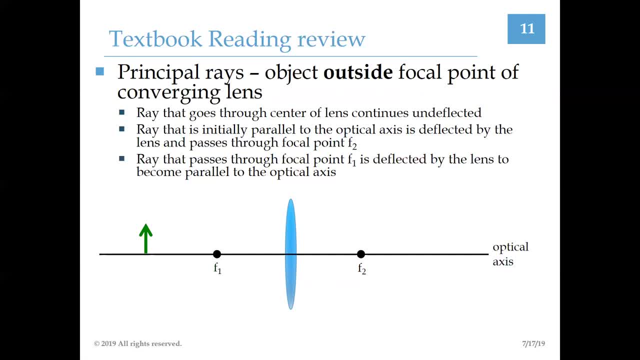 So here are the three principal rays. You've got a ray that goes to the center lens and it's going to continue undeflected. You're going to have a ray that is initially parallel to the optical axis And then, after it encounters the lens, it's going to get deflected and it's going 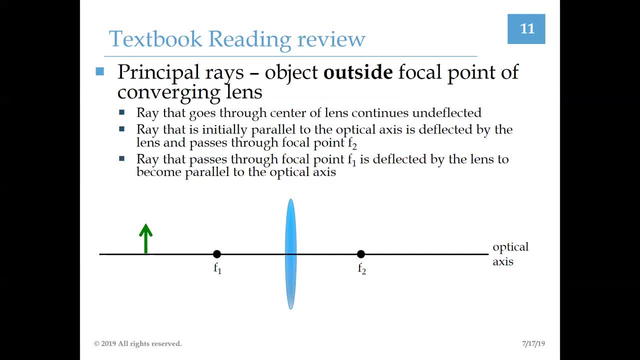 to pass through focal point two, And then a ray that passes through focal point one will be deflected by the lens until it becomes parallel to the optical axis. Now it is worth taking some time here to practice drawing these for yourself. So on Sakai in this. 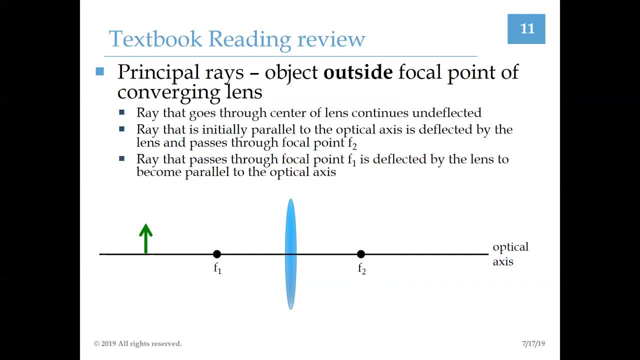 module 19 folder, you can find another PowerPoint slide set called ray tracing, And it basically has a version of this slide here that looks like this, which has none of these rays actually sketched on them, just like you see right now. In a second here I'm going to move forward in this PowerPoint. 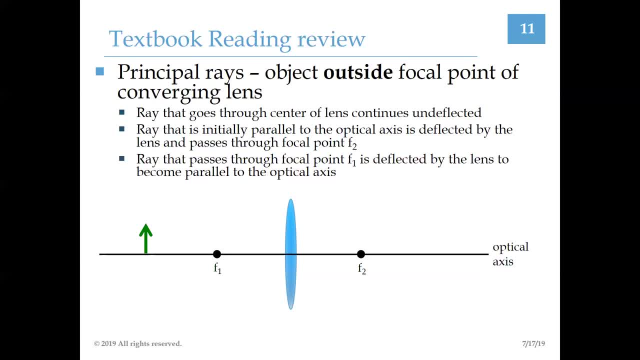 presentation. I'm going to show you what these rays actually look like, But before I do, you really need to try and sketch these out. So I'm going to show you what these rays actually look like And then later on, when you're done, you can take them out, find someGUYs and you can 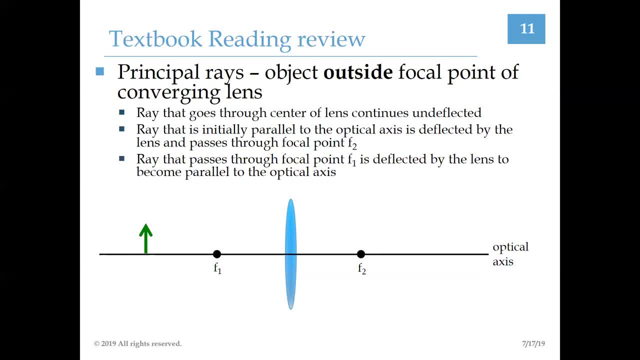 press the Schon quería ded button and align them to your actual slide spends from your jenu Cartel database. So if you need to do that, then you can use the ou salary layer here, but there are a number of different ways you can use the. units for yourself. So go ahead and either copy this figure down on a piece of paper and then try and sketch these three rays or, if you wish, go to that ray tracing PowerPoint slide set, Print off the three slides that are included there and do your sketching right there. 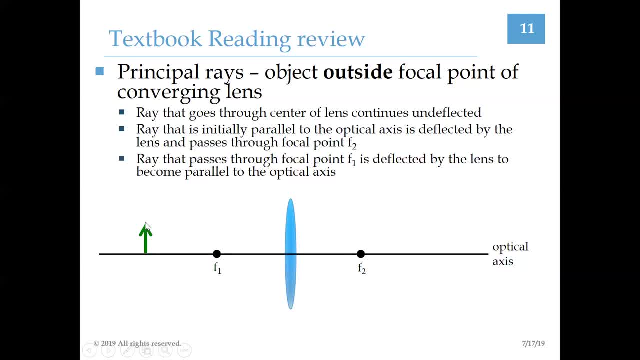 But it's actually really important that you just pause your recording right now. try to draw these. we draw the rays as if they're coming from the very tip of the object, so maybe the very tip of the arrow. You could pick a different point if you wanted to, but make sure all three of those. 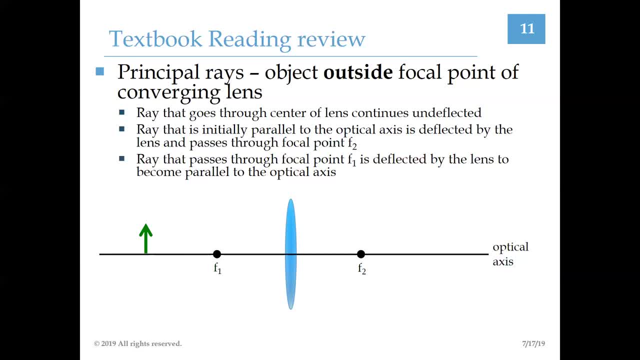 rays are emanating from the same point. Okay, let's go ahead. I'll give you a chance to pause recording right now. Please sketch those three rays. Okay, now that you've had a chance to sketch the rays for yourself, let's see what they look like. Let's see how you did So. boom, here's one. 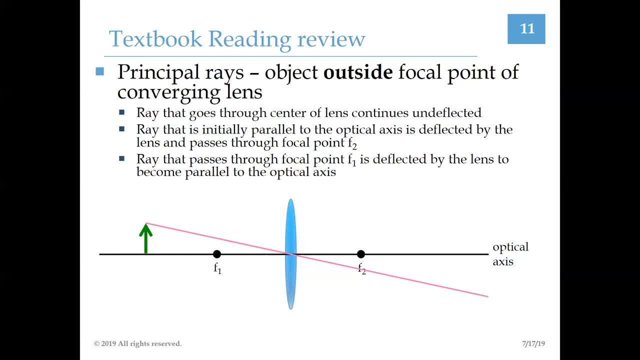 A ray that goes to the center of the lens continues undeflected. So I'm starting right here, at the top of my object. It goes right through the center of the lens and it'll just continue without being bent whatsoever. Let's take a look at our second principal ray. It looks 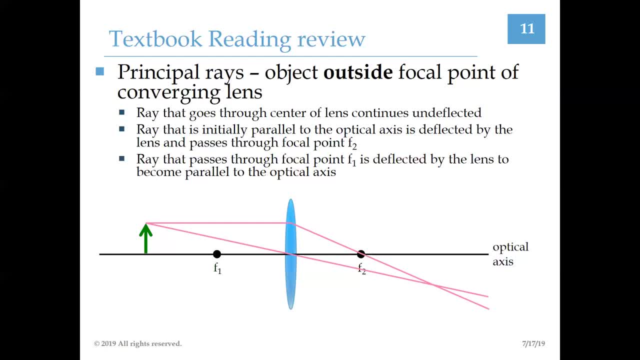 something like this: It's initially parallel to the optical axis, but then, after it hits the lens, it gets deflected such that it now passes through the second focal point. Our third principal ray looks like this, So it came off of the tip of the object. 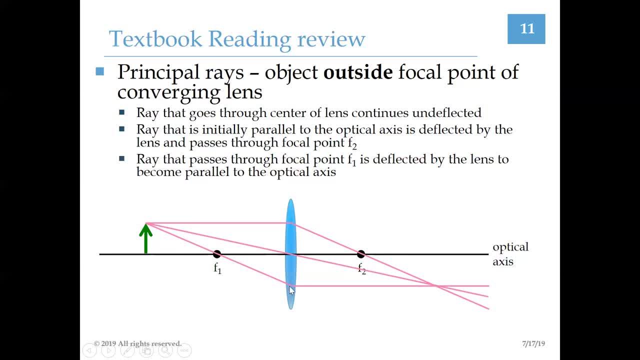 it passed through focal point one and then, once it hit the lens, it got bent such that it is now moving parallel to the optical axis. Those are your three principal rays. Notice something here? All three of those rays appear to come together right here on the right side of the lens. That's where you're going to form. 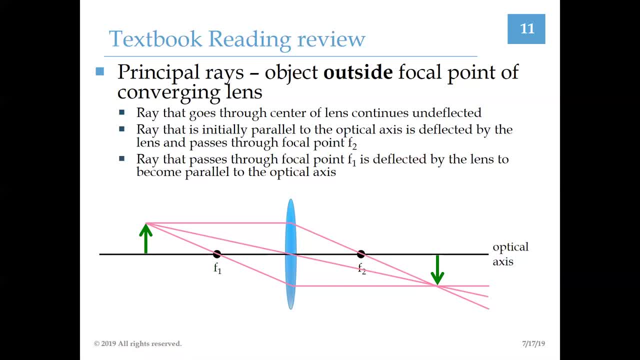 your image. So you form an image of your object right there, where all of those rays appear to come together. Since we had all those rays emanating from the top of the object over here, that means where they all come together. that's where the top of the image is going to appear to. 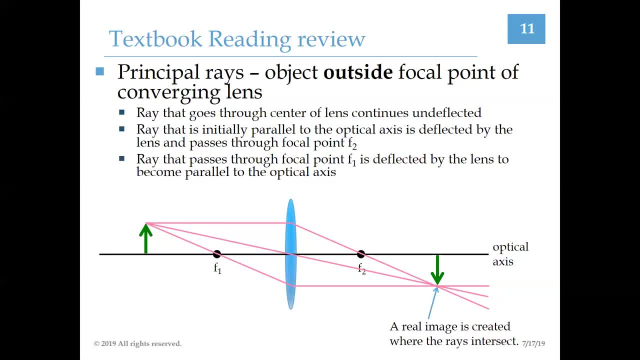 be All right. let me define some things here. That's the image, and we call this the top of the image. What is a real image? Why is it a real image? It's real because the rays of light really intersect there. They're actually coming together and intersecting one another. That's really. 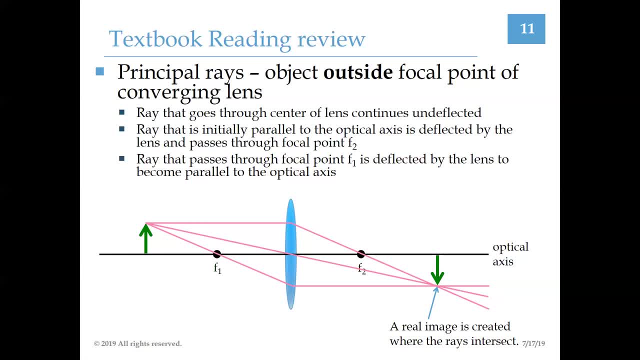 happening And in fact, if you were to put like a screen right here at this point where all the rays are coming together, you would see an image right there. So it's a real image. As I mentioned earlier that distance between the lens and the focal point. 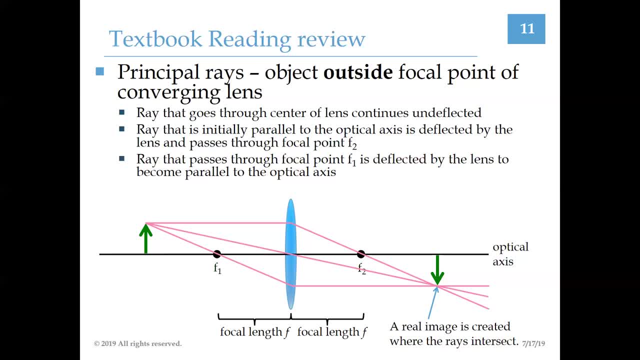 that's called the focal length, And for all the lenses that we're going to consider in physics 115, they're just going to have one focal length. So once you know that focal length, you know the distance to both focal points. Each focal point is one focal length away from the lens. 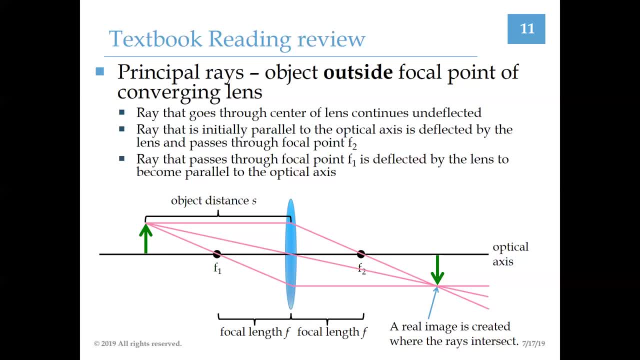 The distance between the object and the lens is very creatively called the object distance And your textbook represents the object distance by the letter F. You can probably guess what the distance between the image and the lens is going to be called. That is called the image distance And your book represents that by the letter S, with a little. 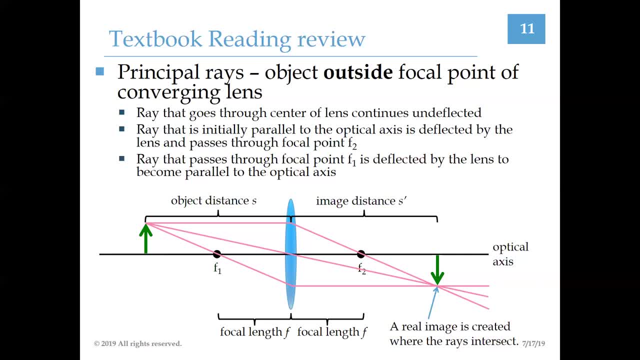 apostrophe by it. We call that S prime. That's your image distance. Notice: focal length, object distance and image distance are all defined relative to the lens. So all of these are expressing some distance. So we can see the distance from the lens. 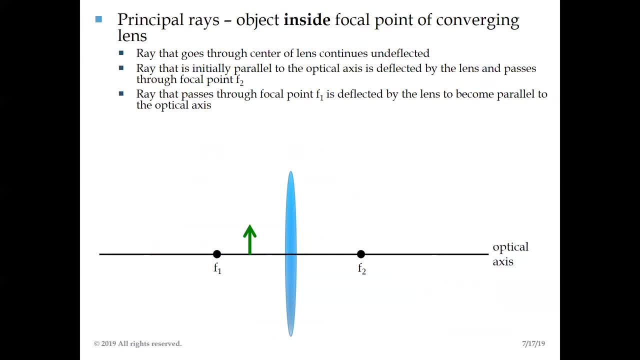 All right, let's take another example here. Same converging lens before Now. the only thing I've done is I've taken my object and I've moved it inside the focal point. My three principal rays are still defined the exact same way, So I still have the same three principal rays as before. At this point, please go ahead, pause your recording and go ahead and please. 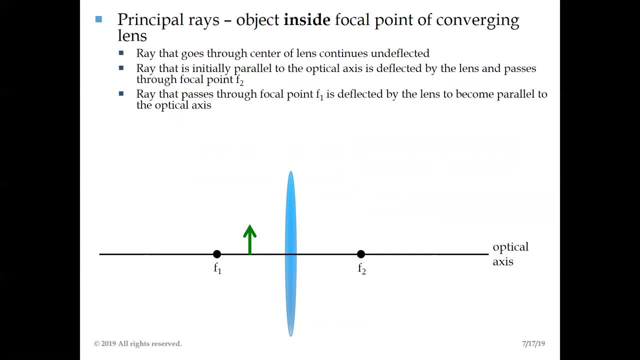 try to sketch these three rays. Now that you've had a chance to sketch the three principal rays for yourself, let's go ahead and see if we can do it all together. So start with the first one. Ray goes to the center and continues undeflected. That's kind of always your freebie. That one's always going to exist, So you might as well always draw that one. It's the easiest one to draw. It's going to exist in every case we talk about Just go ahead and throw it on there. 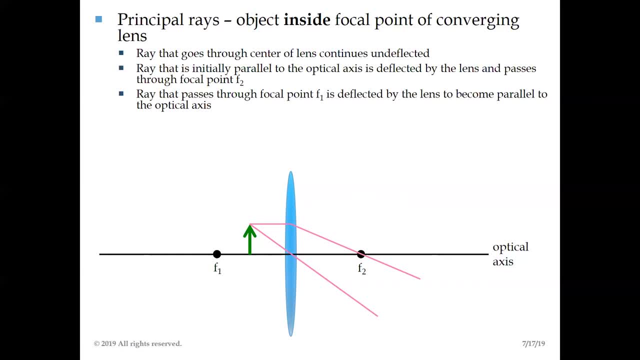 What about the next one? Okay, the next one isn't so bad. Once again, you start out parallel to the optical axis, Then, after you encounter the lens, you get bent, such as you are now passing through the second focal point. 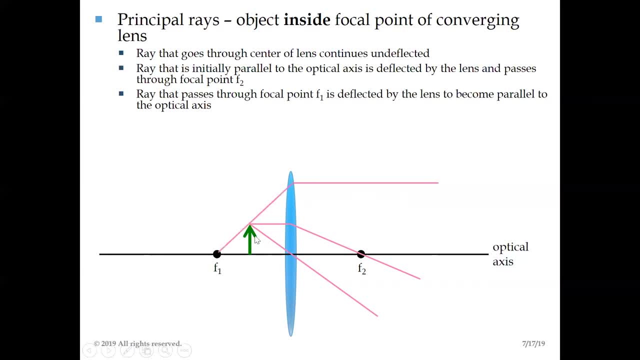 Now what about the third one here? Well, the third one's a little bit gnarly. Now that the object is inside the focal length here you're like: how can the light pass through the focal length one? what you've got to imagine is: imagine you have light coming from the direction that it would. 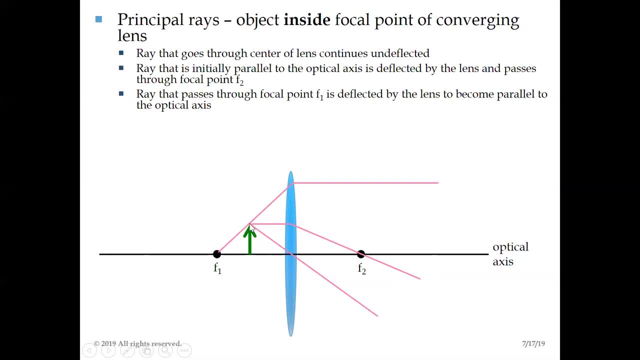 have come in if it had come through focal length one. So really the light ray begins here at the tip of the arrow, but imagine you can draw that line so that it extends back to focal point one and then that beam of light is going to encounter the lens and get bent such that it now comes out. 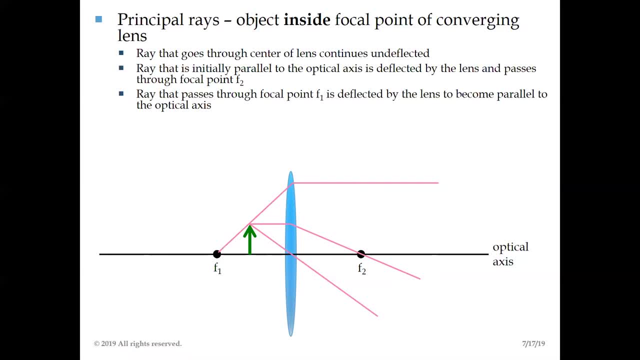 parallel to the lens after passing through the lens. Now look what we have here On the right side of the lens: those three principal rays, unlike the previous case, aren't coming together. They don't converge. So, even though this is a converging lens, you actually will not get rays. 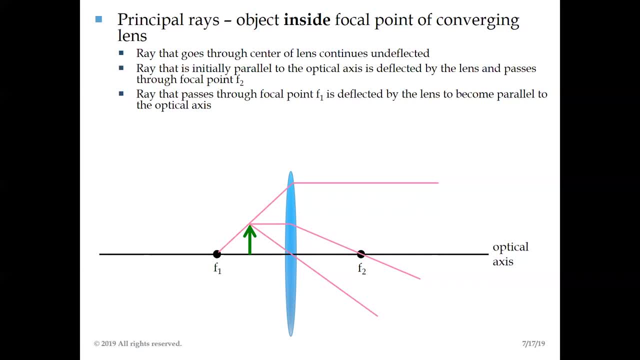 that converge, that actually converge to one another if you place that object inside of the focal point. But now imagine something. Imagine you put your eyeball over here on the right-hand side of the lens. So you put your eyeball over here on the right side of the lens. 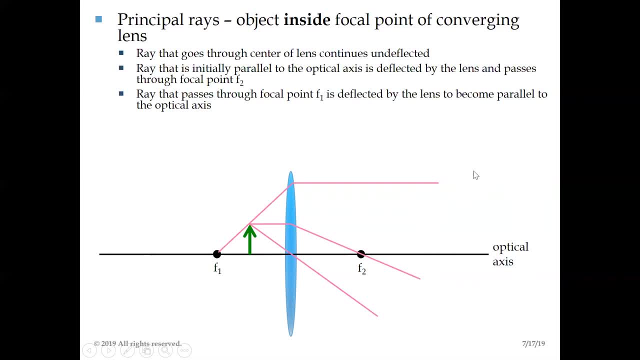 Your brain, your eye is going to intercept all three of these rays, And the thing about your eye and your brain is: your brain doesn't understand that the light was bent. To be fair, my brain doesn't understand that either. It's just a flaw that we all have. 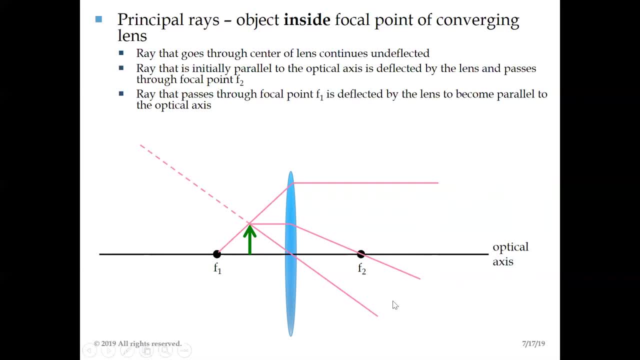 We're just not human beings. And so what happens is your brain thinks that this ray down here actually came from back up here, where I'm showing the dashed line at. It thinks this ray here the one that appeared to go, the one that went through the second focal point. it thinks that 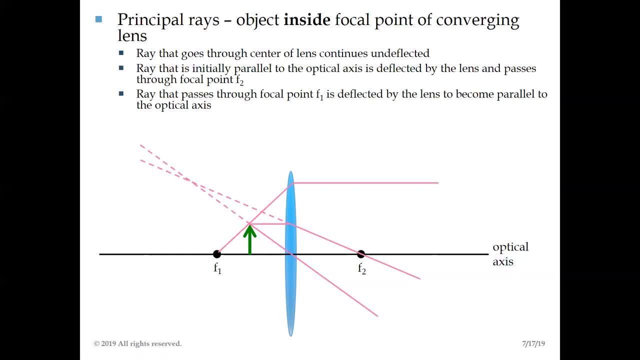 that ray came from back here, where the dashed line is, And the ray that came out parallel. well, your brain thinks it came from over here. something very interesting happens. Your brain thinks that all of those rays converged with one another somewhere back here. So if you were to actually put your eyeball over here on the right, 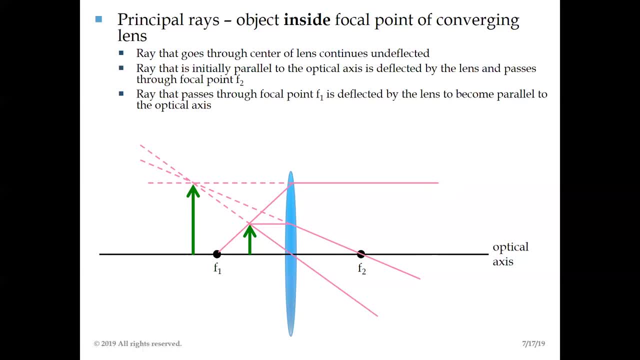 side of your lens, you would see an image. It's what we call a virtual image. It's called virtual because the light rays aren't actually converging at that point where the image forms. Those light rays aren't really coming together there. They don't actually exist there. It's an optical 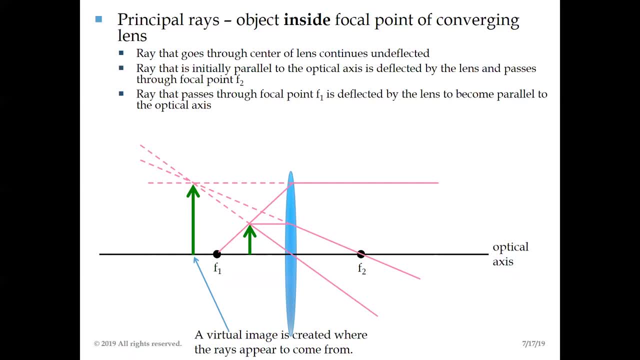 illusion. It's a trick that your brain plays on you, And you might say: well, wait, would I actually see a virtual image? And the answer is yeah, you would. In fact, if you're like me and you wear. 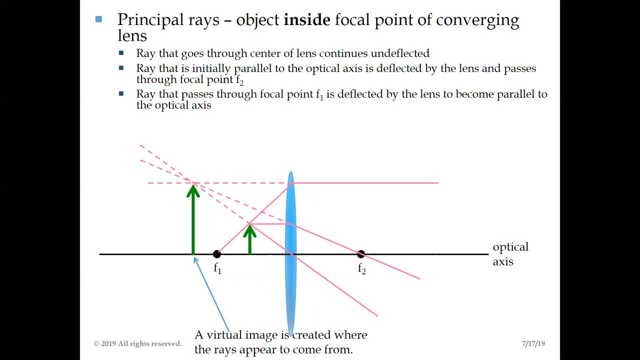 contact lenses or glasses or you've got some sort of something that's correcting your vision. everything you look at is a virtual image. right now, We'll talk about that a little bit more when we talk about vision next time. It's actually a very cool result. 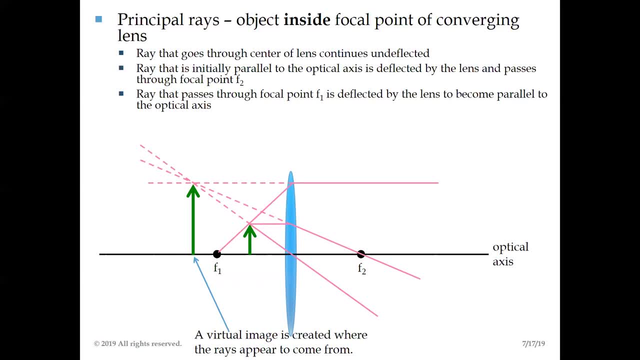 But yeah, most of you have seen virtual images many, many, many times in your life And you just don't realize what you're seeing is virtual. Virtual images look just like real images. They appear to be real to our eyes, But it's important to keep in mind that they're virtual. 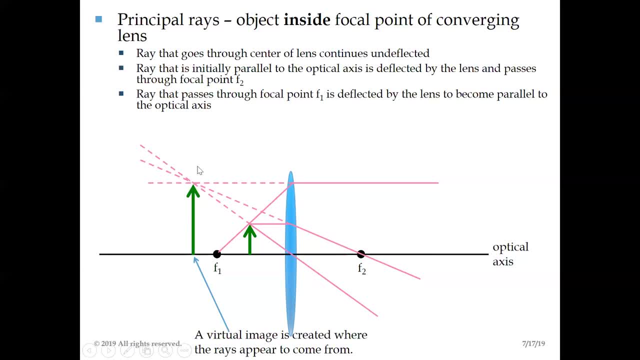 because the light rays aren't actually converging at that point And, in fact, if I were to put a screen right here, I would not see an image on that screen. You only get the image if you put your eyeball to the right here and look. 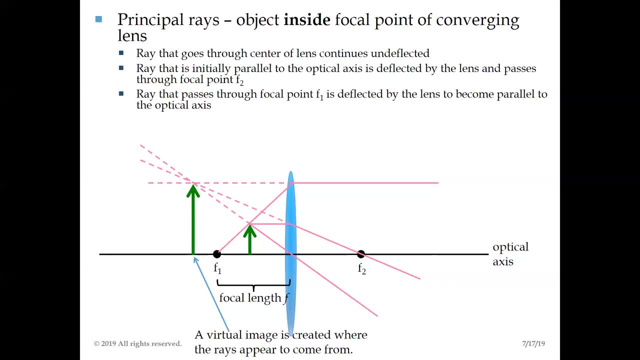 Okay, let's throw in some definitions here. Once again, the focal length is the distance between the lens and the focal point that works on either side of the lens. Once again, your object distance is going to be represented by the letter S here, And it's the distance between your object. 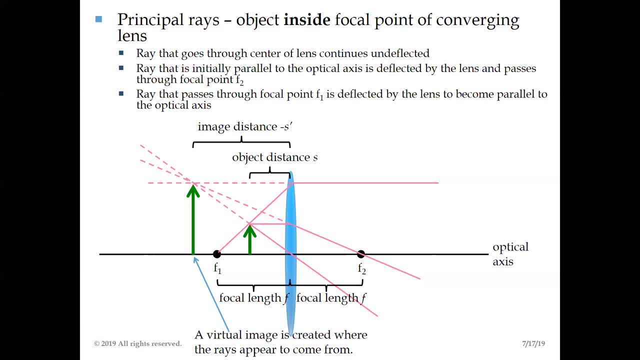 and your lens. Your image distance is once again represented by S prime, And it's the distance between your image and your object And it's the distance between your object and your lens. I'm going to take the vertical symbolism again here. So when we say that your image and your lens, 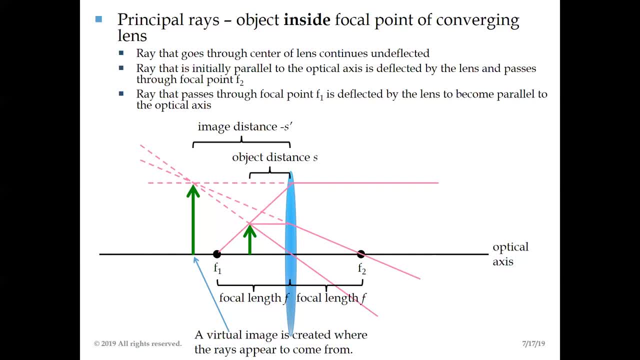 are in a vertical distance, not your image and your object, it's the distance between your image and your lens. One thing to keep in mind here: whenever you have a virtual image, we say the image distance is negative, And likewise if you have a negative image distance, if you do a 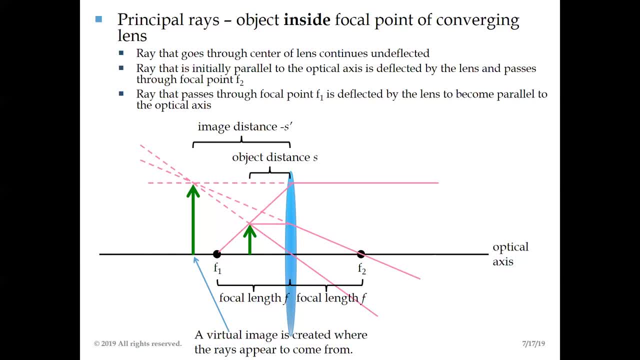 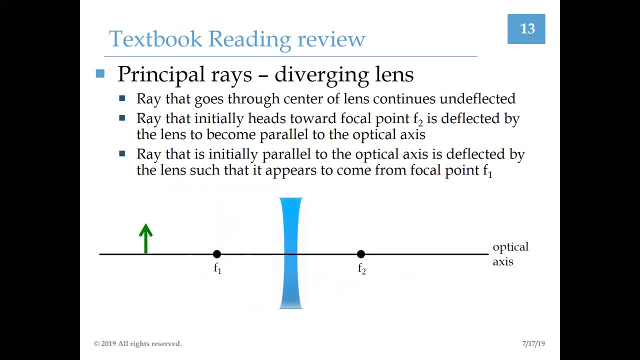 calculation and figure out that your image distance is negative. that means you're dealing with a virtual image. All right, we've got one more case we want to deal with here for ray tracing. This is a diverging lens, And for this one I'm going to go ahead and put the object outside the diverging lens. 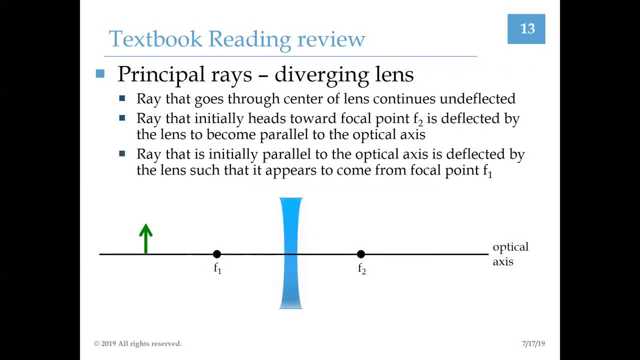 although you'll get the same result if you put the object inside the diverging lens. Here the principal rays are a little bit different than they were for a converging lens, So the first one is the same. You've got a ray that goes through the center and it continues undeflected. 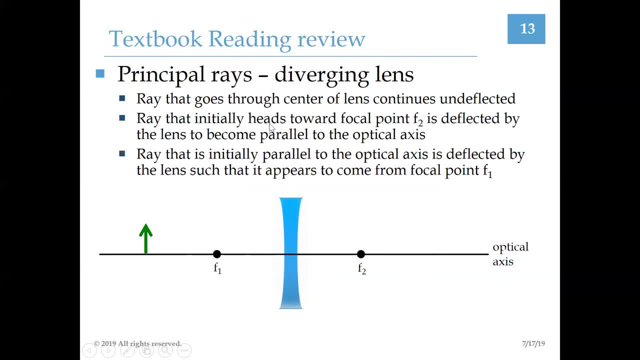 The second one is that you've got a ray that's initially heading towards F2. But then it hits the lens And after hitting the lens it becomes parallel to the optical axis. And the third one is you've got a ray that's initially parallel to the optical axis. 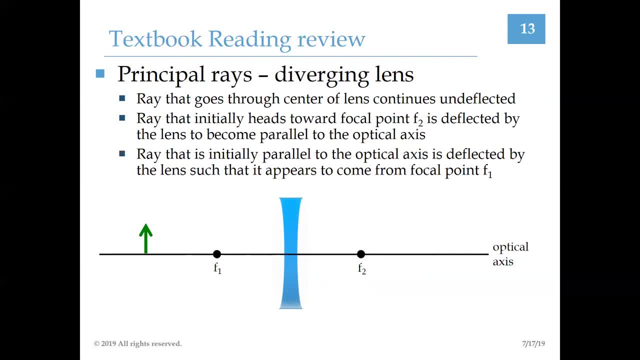 but then it's going to hit the lens and get deflected such that it appears to come from focal point 1.. Okay, with those three rules in mind, please pause your recording and try to sketch those three principal rays for yourself. Again, it's really important. 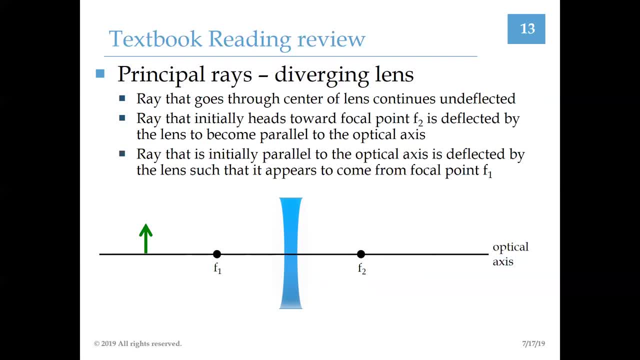 It's important that you try to do this for yourself before we reveal the answer. You don't want to short-circuit the learning process here, So go ahead, pause your recording and try and sketch those three principal rays. Now that you've had a chance to sketch them, let's go ahead and take a look at what they look like. 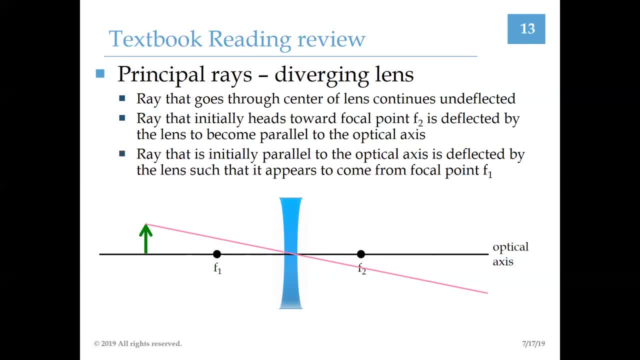 So again, the first one, that's your freebie. Always sketch that for any ray tracing you're always doing. It goes to the center undeflected, Boom, Easy. What about the next one? Well, the next one is a beam of light that starts as if it were heading towards F2.. 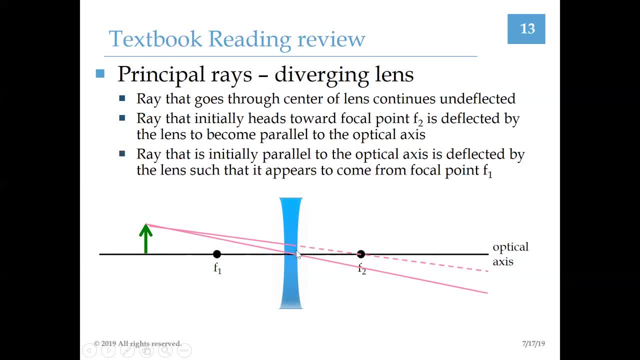 So once I hit the lens here, I turn it into a dashed line because it doesn't actually go through F2, because it hits the lens and then boom, it gets bent such that it comes out parallel to the optical axis. 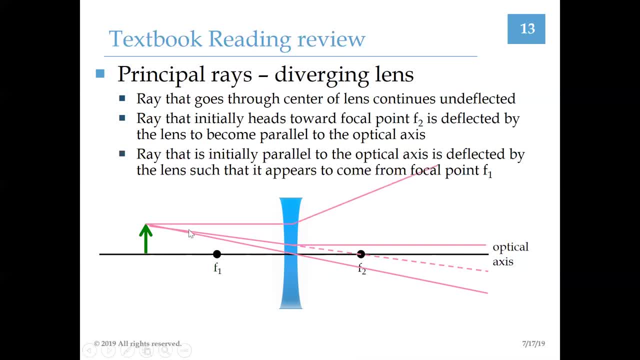 The third one was initially parallel to the optical axis, but then it hits the lens and it gets bent such that it appears to be coming away from F1. So imagine extending this line back to F1. That's what the dashed lines are representing here. 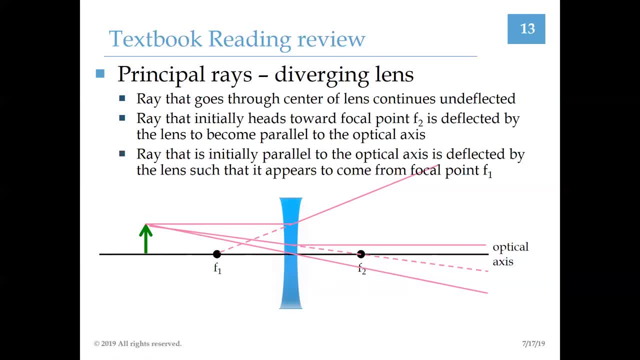 That's telling you the direction in which the light ray is moving, now that it's passed through the lens and it's on the other side. So I'm going to get rid of those dashed lines here, just to clean this up a little bit. 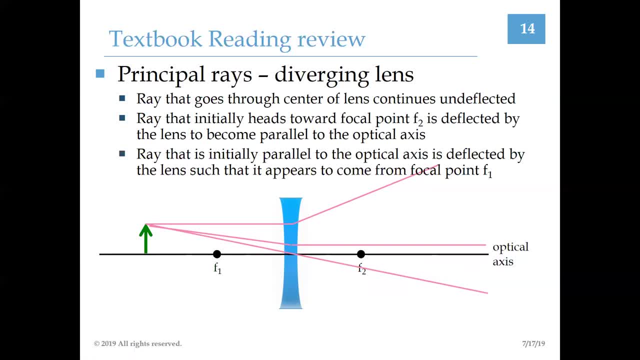 As you can see here, as you might have expected, a diverging lens actually produces rays that diverge from one another, So they're not converging. You're not going to produce a real image, But once again, if I put my eyeball on the right side here, 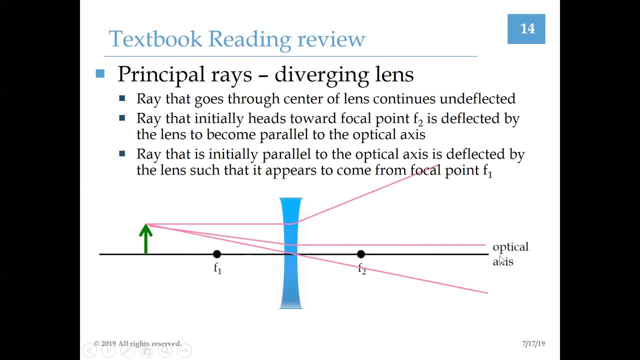 on the opposite side of the lens, from the object. my brain is going to think, for example, that this top ray came from back here. It's going to think that this middle ray came from back here and the one that passed through the center undeflected. 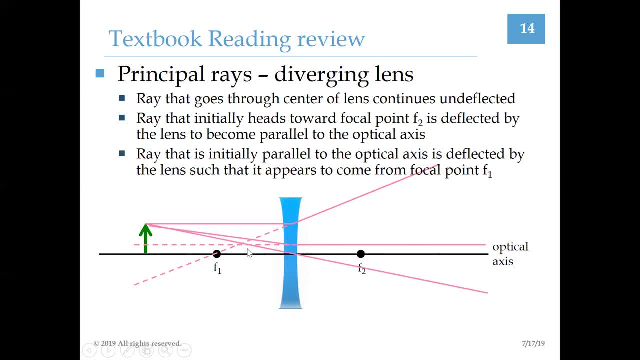 it's going to think it came from where it did actually, And so notice those three rays, my brain is going to think, converge back here On the same side of the lens as the object, So I'll form an image right there. 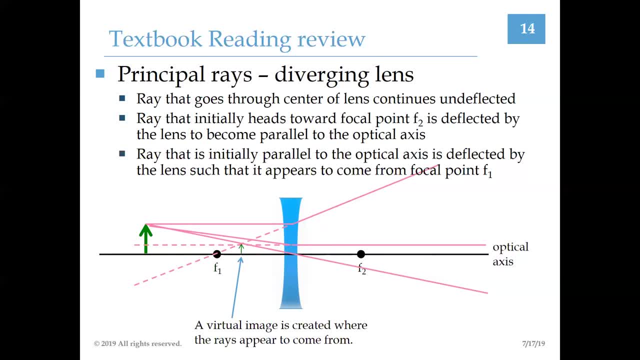 It's a virtual image. Again, it's virtual because the light rays aren't really coming together there. This is an optical illusion, It's a trick. my brain is playing on me, But I swear if you put your eyeball on the right side of this lens here. 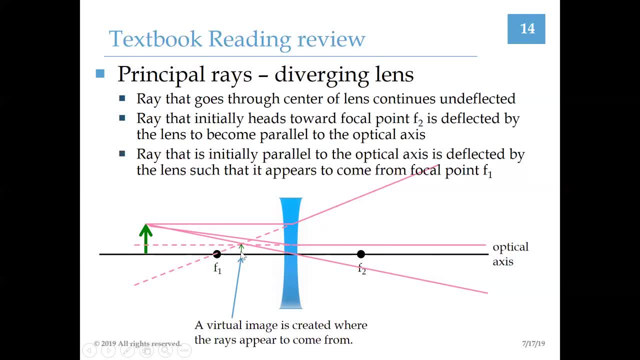 you would see that image. You would not see the object, You would see the image of the object. There's our focal lengths. The magnitude, the absolute value of the focal length tells you how far away each focal point is from the lens. 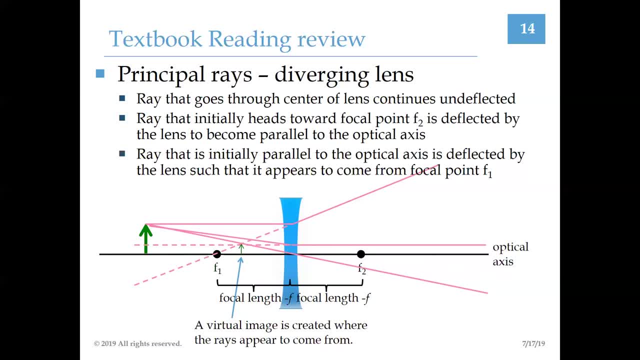 But just keep in mind, since this is a diverging lens, we will say that the focal length is negative. So if I gave you a diverging lens, I might say, for example, the focal length is negative three centimeters. That would tell you that each focal point is three centimeters away from the lens. 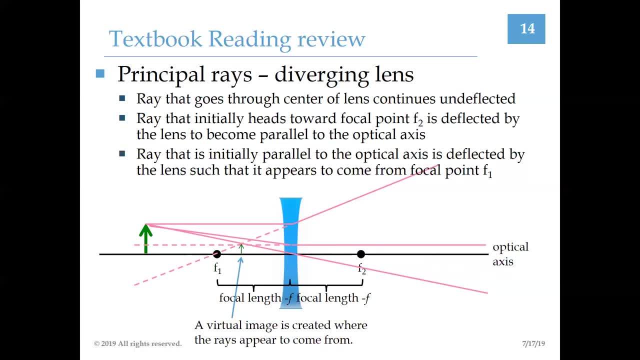 But the negative, the negative sign there tells you it's a focal length. So if I gave you a focal length, I might say, for example: the focal length is negative three centimeters. But if I gave you a focal length, I might say, for example: 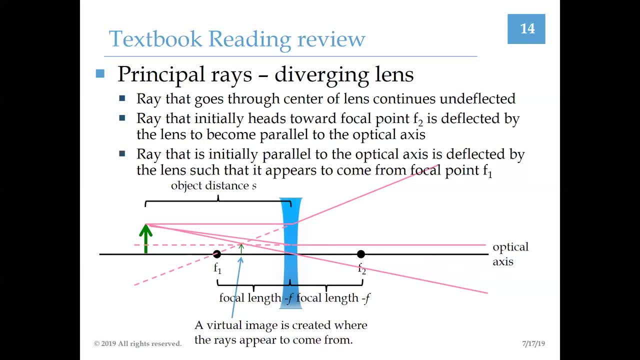 the focal length is negative three centimeters. It's a diverging lens. Object distance S is the distance between the object and the lens. The image distance S, prime is the distance between the image and the lens And, once again, since your image is on the, it's going to be virtual. we're going to say 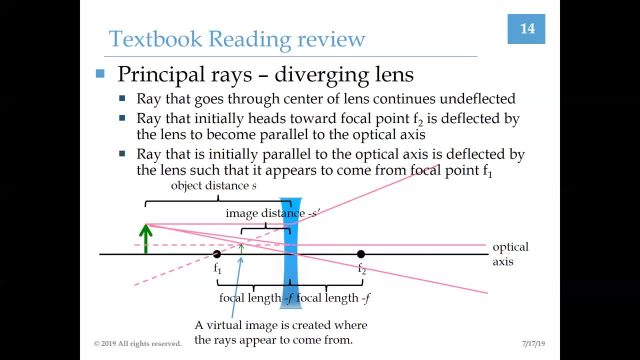 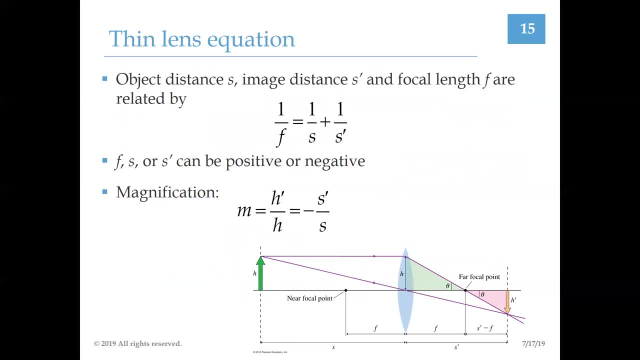 that your image distance is negative. So negative image distances correspond to virtual images. So ray tracing is a really powerful tool. Another powerful tool that you're going to need for geometrical optics: are these equations right here? These are basically the only two equations, in addition to maybe, Snell's law, that you're 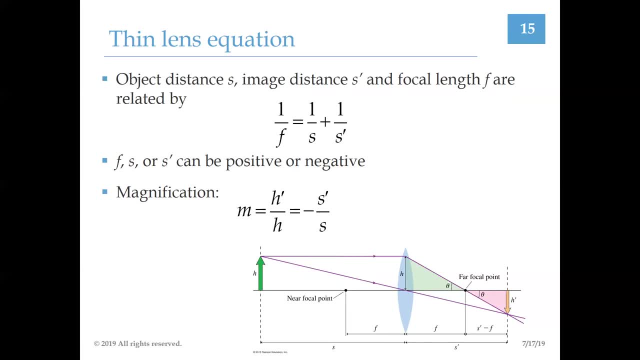 going to need One is called the thin lens equation, also called the lensmaker's equation. Some people have called it the lenscrafter's equation before. It's not lenscrafter's. The lenscrafter's store, as you see in the mall, has not copyrighted this equation. 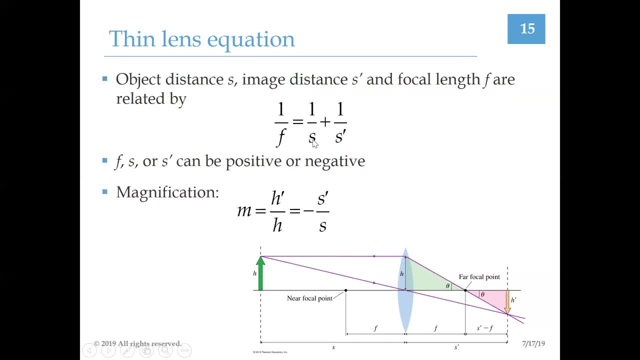 But this equation here relates the focal length, the image distance S prime and the object distance S together. So one over the focal length will equal one over the object distance plus one over the image distance. So if I know any two of these I can figure out the third. 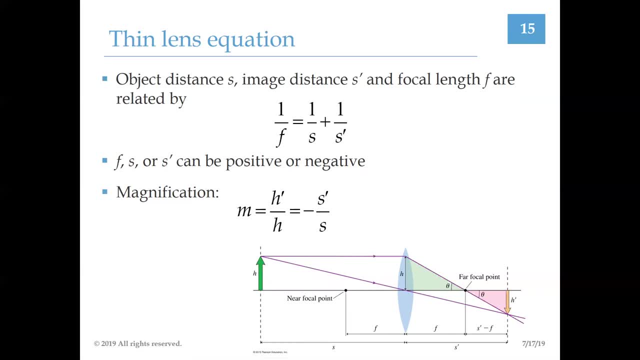 That's really useful. The other thing that we have to reckon with is magnification. So the magnification is defined as basically the height of your image divided by the height of your object, And you can go through some geometrical proofs here What this figure down here is showing. 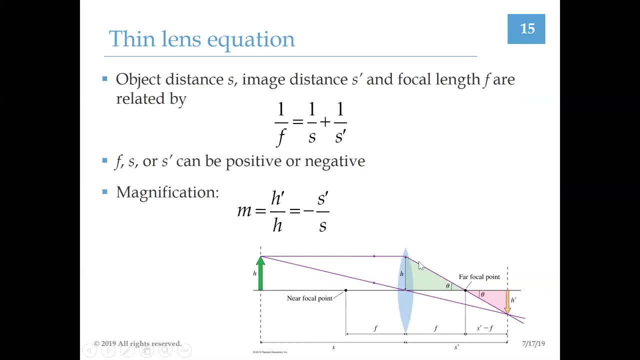 Don't worry about going through those geometrical proofs, But you can use them to show that the magnification is also equal to negative S, prime over S, So negative of the image distance over the object distance. Now, before we wrap this up, I do want to put out a couple words of warning here. 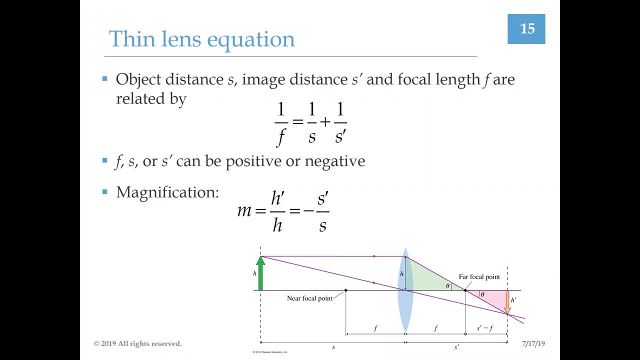 So first of all, keep in mind that these quantities- F and S prime and S prime and S prime, for example- could be positive or negative. So make sure in these equations you insert that negative sign with it. So, for example, if I'm calculating a magnification and my image distance is negative, I would 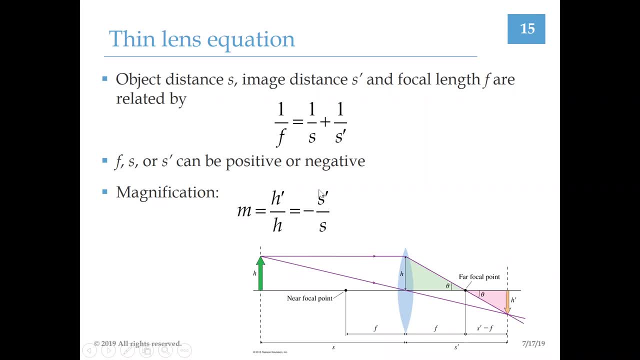 have negative and then S prime itself is negative, So I'd have two negatives. Those two negatives would cancel out and give me a positive. So if you've got a negative sign associated with one of these quantities, make sure you insert that negative sign with the quantity. 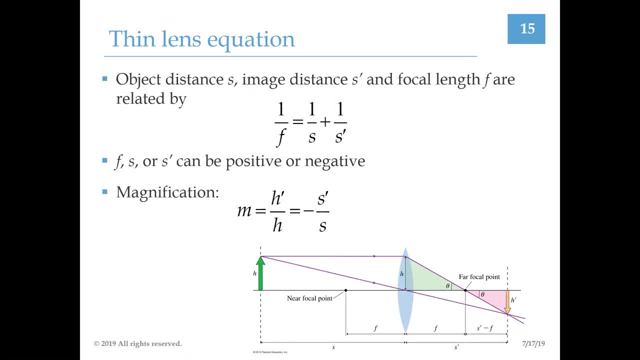 Okay, So that's what we're going to do when we use these equations. The other thing to keep straight is what the different negative signs represent. A negative focal length represents a diverging lens. A negative image distance represents a virtual image, And a negative magnification represents an image that's inverted relative to the object.